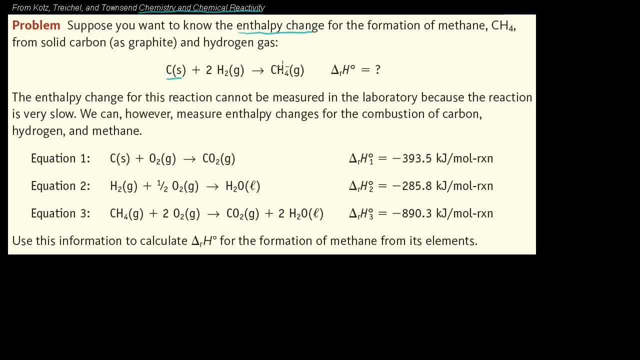 right there- and hydrogen gas. So we want to figure out the enthalpy change of this reaction. How do we get methane? How much energy is absorbed or released when methane is formed from the reaction of solid carbon as graphite and hydrogen gas? 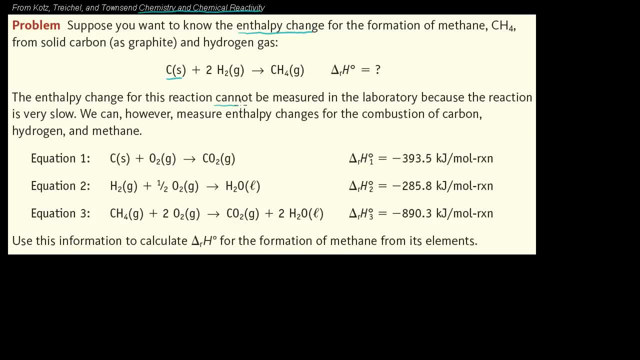 So they tell us the enthalpy change for this reaction cannot be measured in the laboratory because the reaction is very slow. So normally if you could measure it you would have this reaction happening and you would kind of see how much heat or what's the temperature change of the 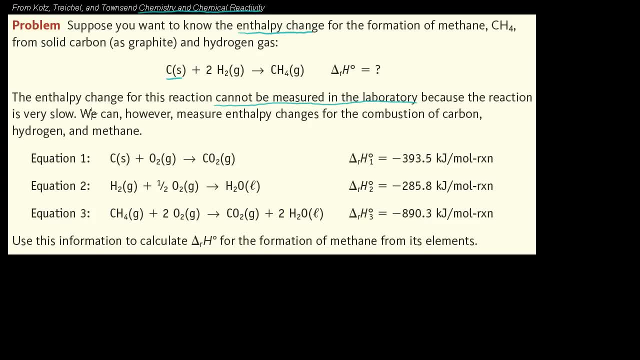 surrounding solution. Maybe this is happening so slow that it's very hard to measure that temperature change, or you can't do it in any meaningful way. We can, however, measure enthalpy changes for the combustion of carbon hydrogen and methane. 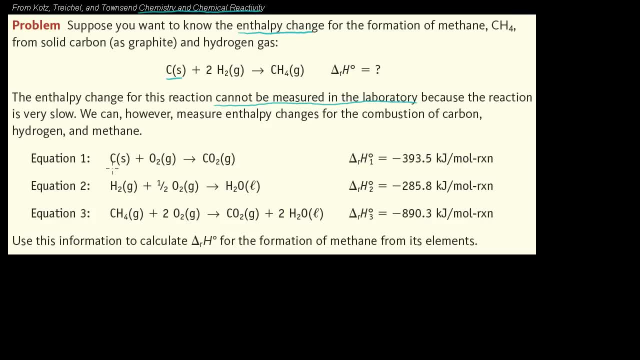 So they're giving us the enthalpy changes for these combustion reactions- combustion of carbon, combustion of hydrogen, combustion of methane- and they say: use this information to calculate the change in enthalpy for the formation of methane from its elements. 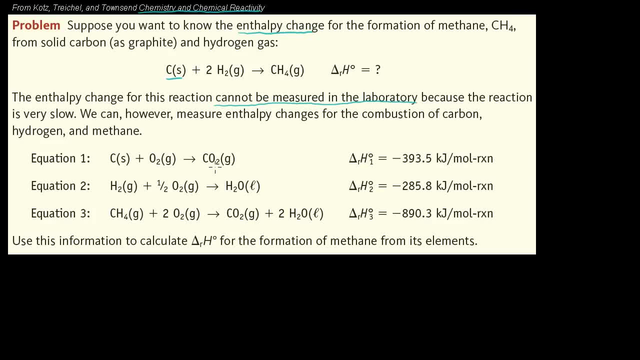 So anytime you see this kind of situation where they're giving you the enthalpies for a bunch of reactions and they say, hey, we don't know the enthalpy for some other reaction and that other reaction seems to be made up of similar things, your brain should immediately 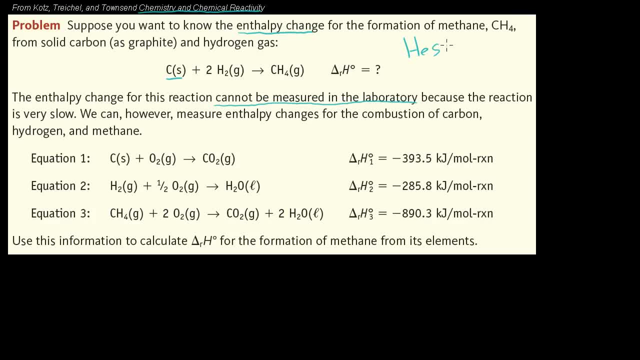 say, hey, maybe this is a Hess's Law problem, And all Hess's Law says is that if a reaction is the sum of two or more other reactions, then the change in enthalpy of this reaction is going to be the sum of the change in. 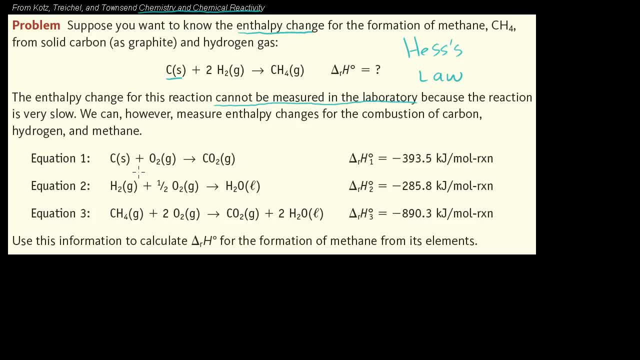 enthalpies of those reactions. Now, when we look at this- and this tends to be the confusing part- is: how can you construct this reaction out of these reactions over time? OK, OK, So we're going to start with methane, And what I like to do is just start with the end product. 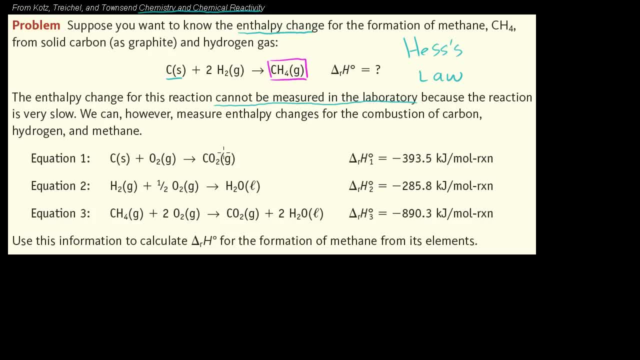 So I like to start with the end product, which is methane in a gaseous form, And when we look at all of these equations over here, we have the combustion of methane, So this actually involves methane. So let's start with this. 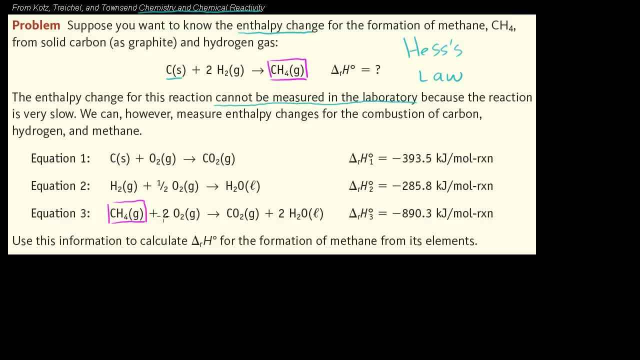 But this one involves methane as a reactant, not a product. But what we can do is just flip this arrow and write it as methane as a product. So if we just write this reaction and we flip it, so now we have carbon dioxide gas. 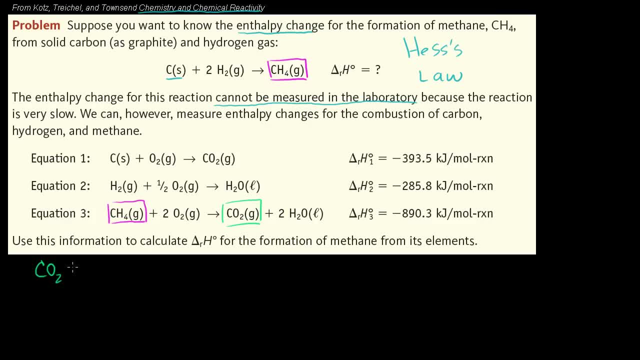 Let me write it down here: Carbon dioxide, gas plus- I'll do this in another color- plus two waters plus two, if we're thinking of these as moles, or two molecules of water. you could even say two molecules of water in its liquid state. 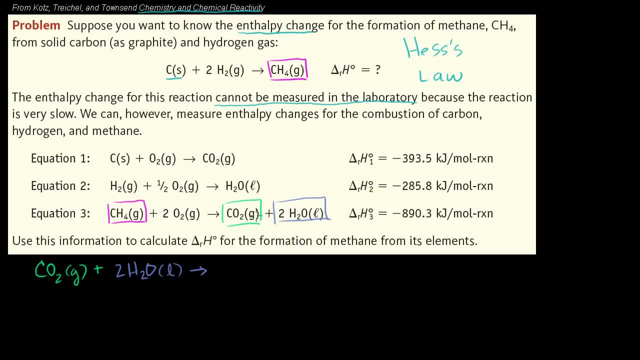 That can. I guess you can say this would not happen spontaneously because it would require energy. But if we just put this in the reverse direction, OK, If you go in this direction you're going to get two waters. I'll do that in a different- or two oxygens. I. 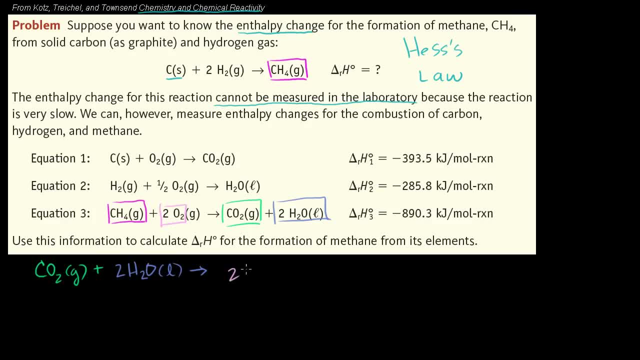 should say: I'll do that in this pink color. So two oxygens plus, and that's in its gaseous state, plus a gaseous methane, CH4- in a gaseous state, And all I did is I wrote this third equation. 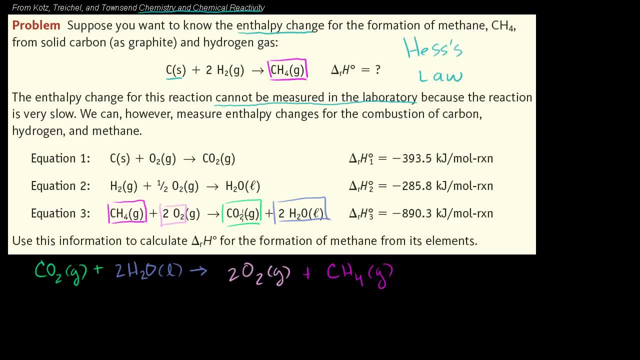 But I wrote it in reverse order. I'm going from the reactants to the product. So if I'm going from the, when you go from the product to the reactants, it will release 890.3 kilojoules per moles of. 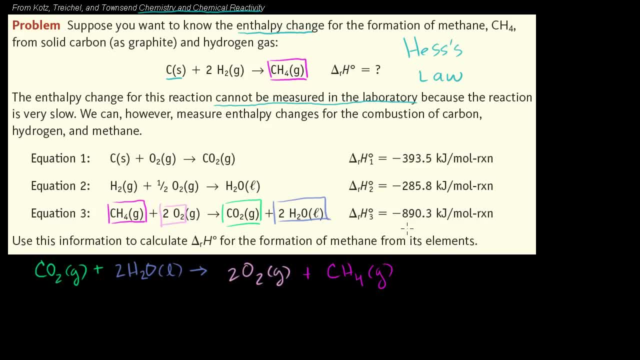 the reaction going on, But if you go the other way it will need 890 kilojoules, So the delta H here. I'll do this in a neutral color, So the delta H of this reaction right here is going to be the 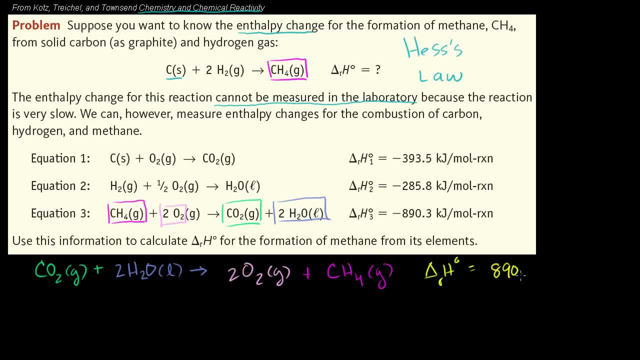 reverse of this. So it's positive 890.3.. OK, It's going to be kilojoules per mole of the reaction. All I did is I reversed the order of this reaction right there. The good thing about this is I now have something that at. 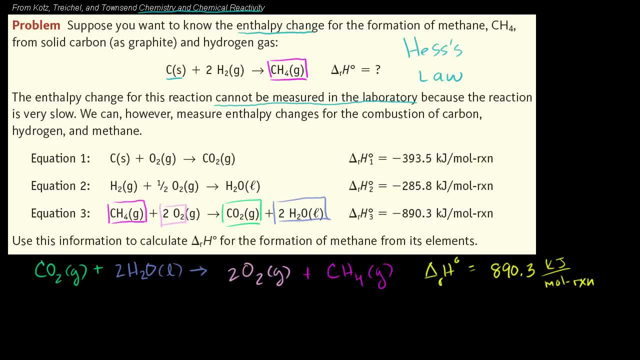 least ends up with what we eventually want to end up with. This is where we want to get. This is where we want to get eventually. Now, if we want to get there eventually, we need to, at some point, have some carbon dioxide, and we have to have at. 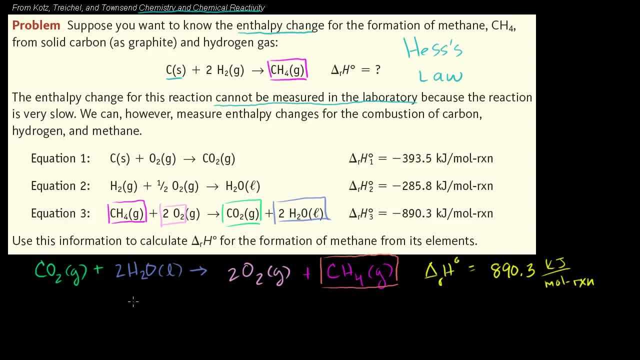 some point some water to deal with. So how can we get carbon dioxide and how can we get water? Well, these two reactions right here. This combustion reaction gives us carbon dioxide, This combustion reaction gives us water. So we could just rewrite those. 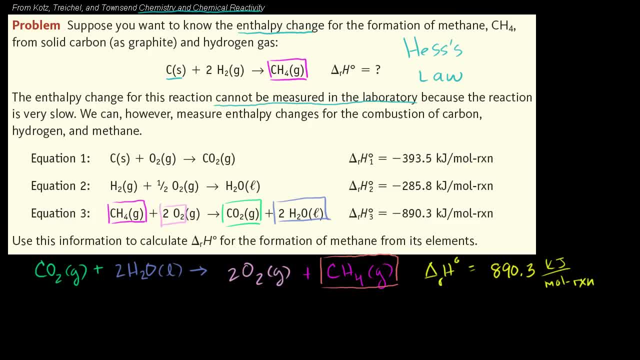 Let me just rewrite them over here And I will use some colors. So if I start with graphite, carbon in graphite form, So carbon in its graphite form plus, I already have a color for oxygen, plus oxygen in its gaseous state. 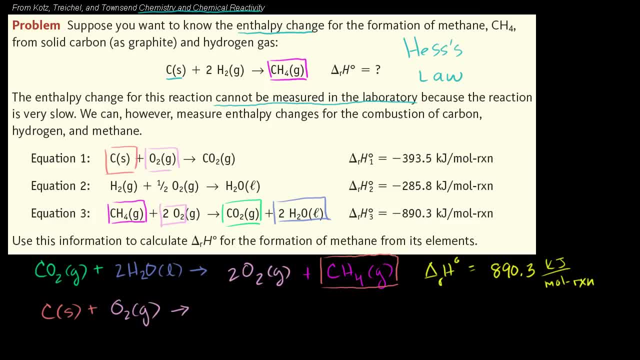 It will produce carbon dioxide in its gaseous form and this reaction. So when you take the enthalpy of the carbon dioxide and from that you subtract the enthalpy of these reactants, you get a negative number, Which means this had a lower enthalpy, which means energy. 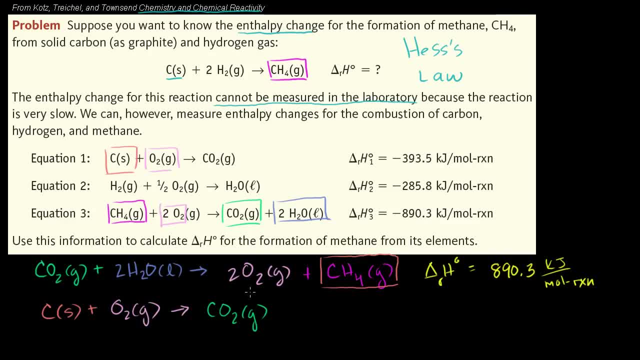 was released because there's now less energy in the system right here. So this is essentially how much energy was released. Now, this is essentially how much energy was released, which is released, But our change in enthalpy here, our change in enthalpy. 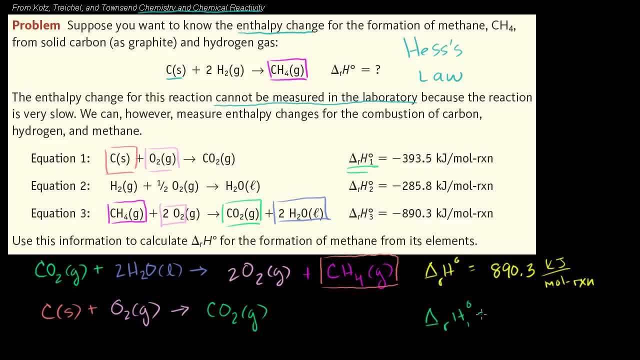 of this reaction right here. that's reaction one. I'll just rewrite it: Minus 393.5 kilojoules per mole of the reaction occurring. So the reaction occurs a mole times. This would be the amount of energy that's essentially released. 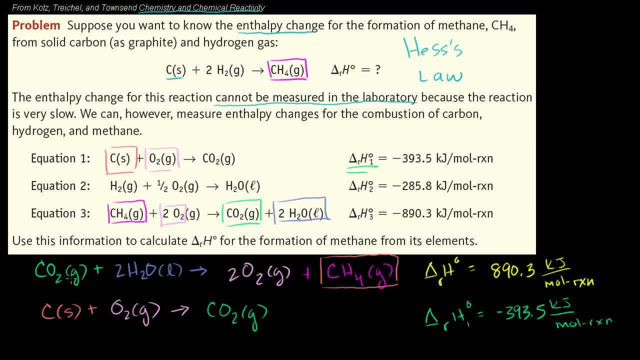 This is our change in enthalpy, So if this happens, we'll get our carbon dioxide, And so we would release this much energy and we'd have this product to deal with. But we also now need our water, And this reaction right here gives us. 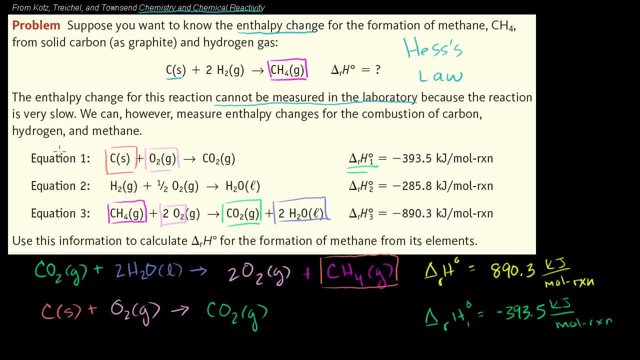 our water, the combustion of hydrogen. So we have, and I haven't done hydrogen yet. so let me do hydrogen in a new color. That's not a new color, Let me do blue. So right here you have hydrogen gas. 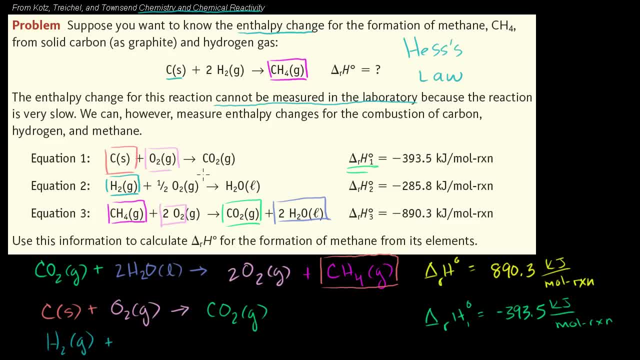 I'm just rewriting that reaction: Hydrogen gas plus 1.5.. O2. Pink is my color for oxygen. 1.5 O2 gas will yield. will give us some water, Will give us H2O, Will give us some liquid water. 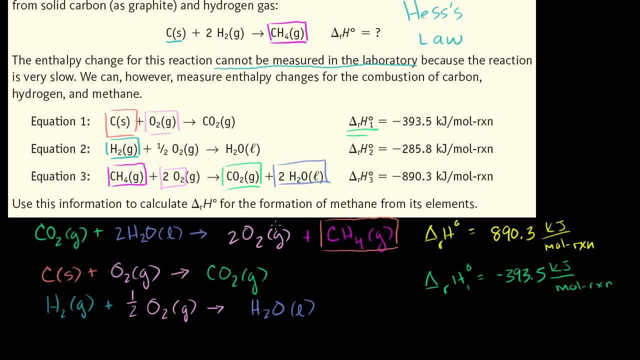 Now, before I just write this number down, let's think about whether we have everything we need To make this reaction occur, because this gets us to our final product. this gets us to the gaseous methane. we need A mole, or we can even say a molecule, of carbon dioxide. 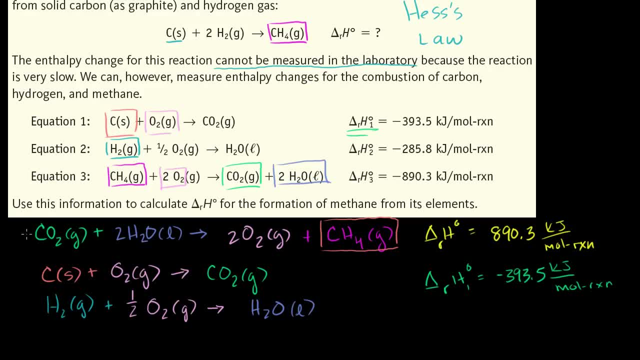 And this reaction gives us exactly one molecule of carbon dioxide. So that's a check, And we need two molecules of water. Now, this reaction only gives us one molecule of water, So let's multiply both sides of the equation to get two molecules of water. 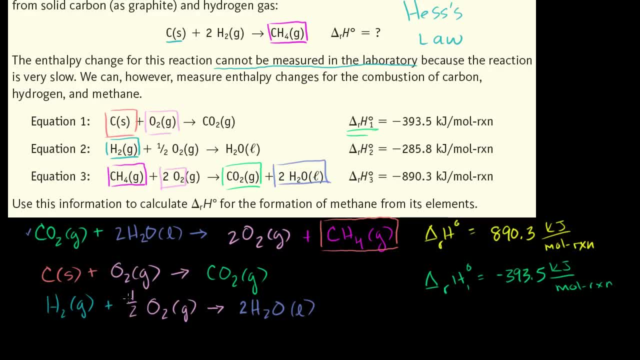 So this is a 2. We multiply this by 2, so this essentially just disappears. You multiply 1.5 by 2, you just get a 1 there And then you put a 2 over here. So I just multiplied this second equation. 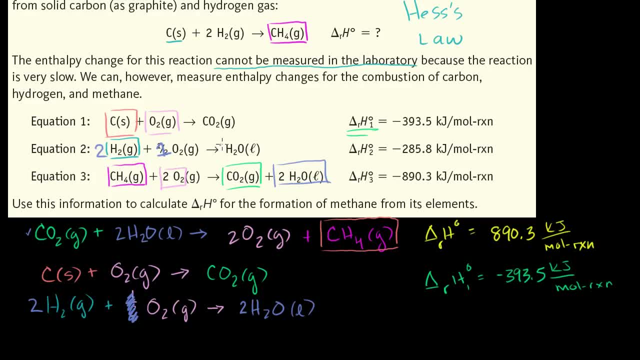 by 2.. So I just multiplied this. This becomes a 1.. This becomes a 2.. And if you're doing it, twice as much of it because we multiplied it by 2, the delta H, now the change in enthalpy of the reaction. 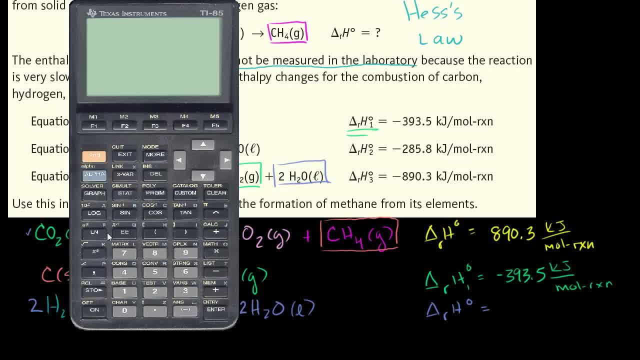 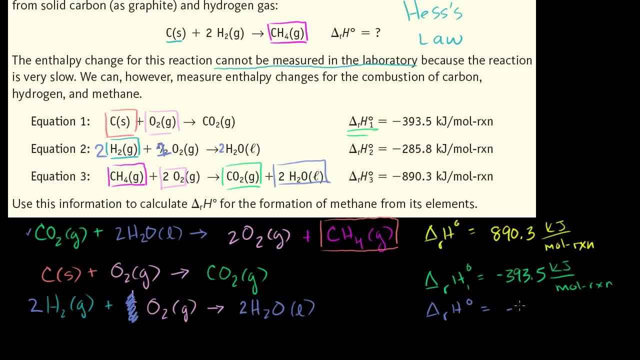 is now going to be twice this. Let's get the calculator out. It's going to be negative 285.8 times 2.. Because we just multiplied the whole reaction times 2.. So negative 571.6.. So it's negative 571.6 kilojoules per mole of the reaction. 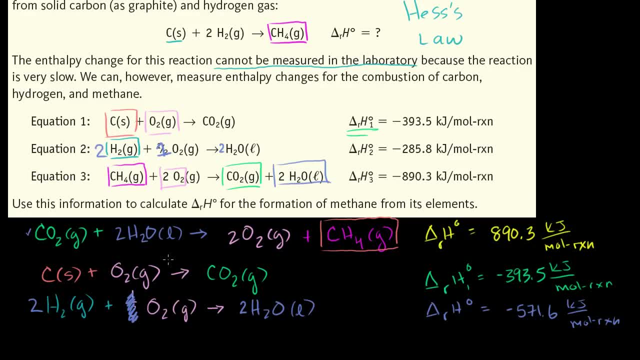 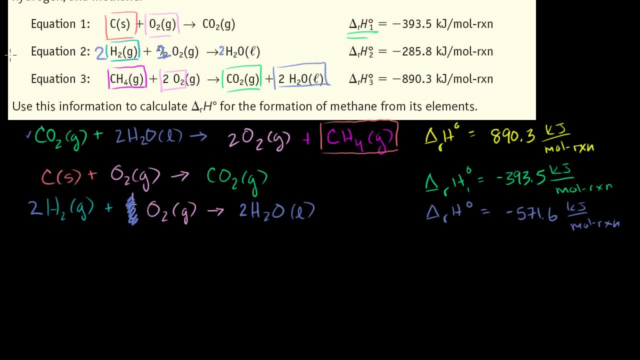 Now let's see if the combination, if the sum of these reactions actually is this reaction up here. And to do that, actually let me just copy and paste this top one here, Because that's kind of the order that we're going to go in. 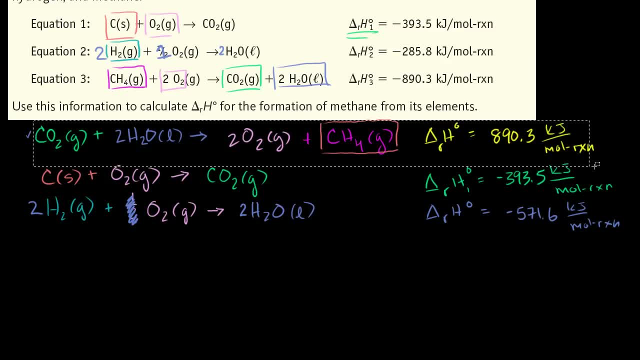 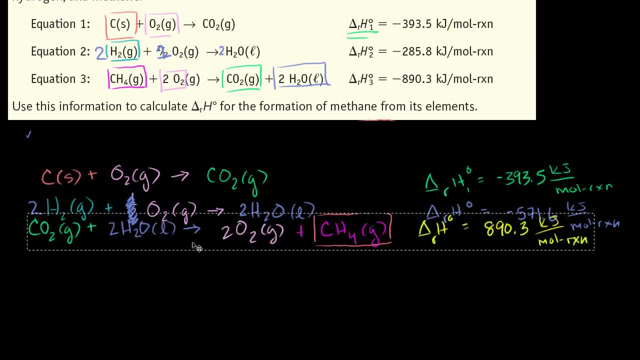 You don't have to, but it just makes it hopefully a little bit easier to understand. So let me just copy and paste this. Actually, I could cut this. Let me cut and paste it, Cut and then let me paste it down here, that first one: 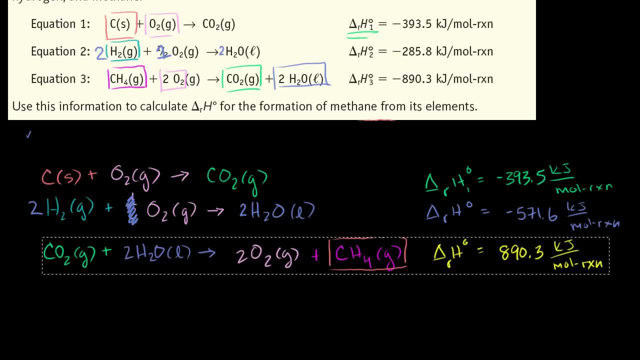 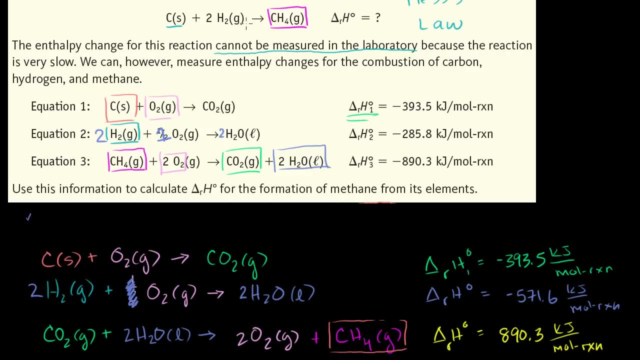 And let's see now what's going to happen And to see whether the sum of these reactions really does end up being this top reaction right here. let's see if we can cancel out reactants and products, Or let's see what would happen. 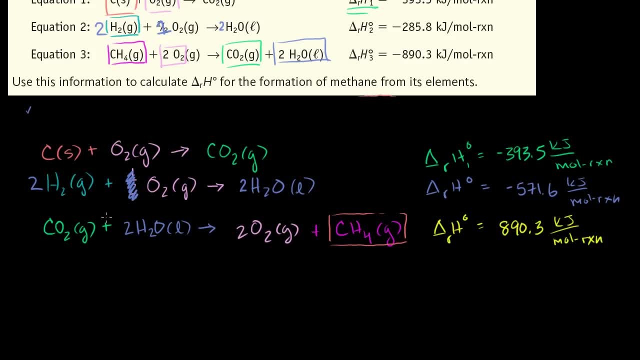 So this produces carbon dioxide, but then this mole or this molecule of carbon dioxide is then used up in this last reaction. So this produces it, This uses it. So those cancel out. Let me do it in the same color, So it's in this green. 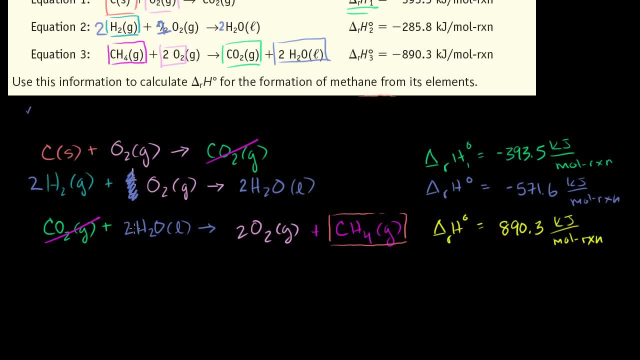 This reaction produces it. This reaction uses it. Now this reaction right here produces the two molecules of water. And now this reaction down here- I want to do that- same color. There's two molecules of water. Now this reaction down here uses: 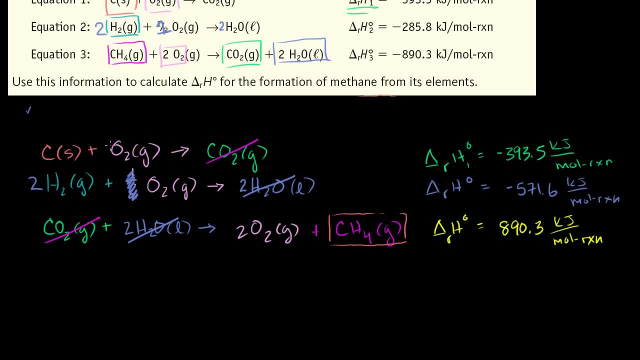 those two molecules of water. Now this reaction right here, it requires one molecule of molecular oxygen. This one requires another molecule, One molecule of molecular oxygen. So these two combined are two molecules of molecular oxygen. So those are the reactants. 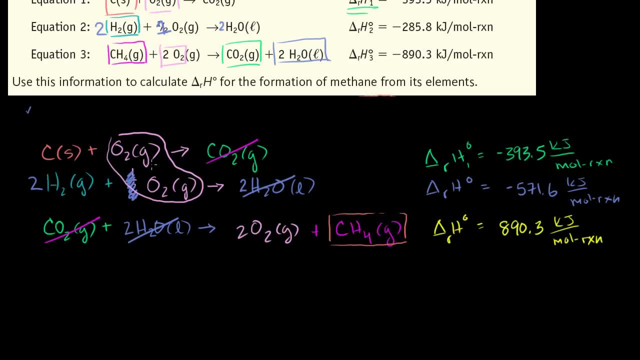 And in the end those end up as the products of this last reaction. So those actually, they go into the system and then they leave out the system or out of the sum of reactions unchanged. So they cancel out with each other. 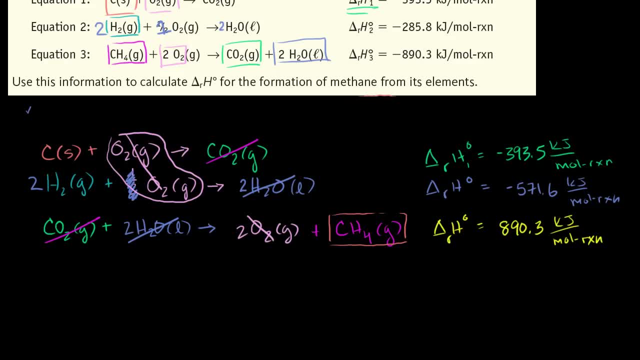 So we could say that and that we cancel out. And so what are we left with? What are we left with in the reaction? Well, we have some solid carbon as graphite, plus two moles or two molecules of hydrogen. 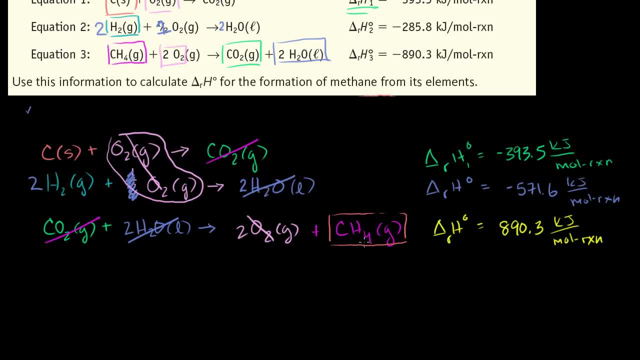 molecular hydrogen yielding. All we have left on the product side is some methane. So it is true that the sum of these reactions is exactly what we want. All we have left on the product side is the graphite, the solid graphite, plus the molecular hydrogen, plus the gaseous hydrogen. 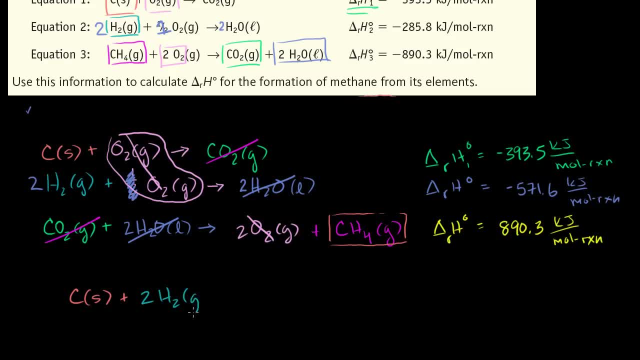 Do it in that color Plus two hydrogen gas, And all we have left on the product side is some methane. All we have left on the product side is the methane. All we have left is the methane in the gaseous form. 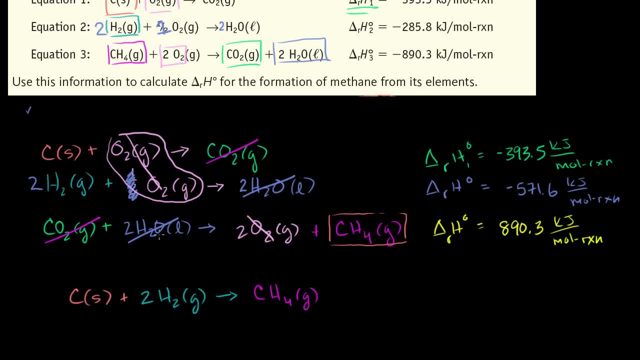 So it is true that the sum of these reactions- remember, we had to flip this reaction around and change its sign and we had to multiply this reaction by two so that the sum of these becomes this reaction that we really care about. So, since this is the sum of these reactions, 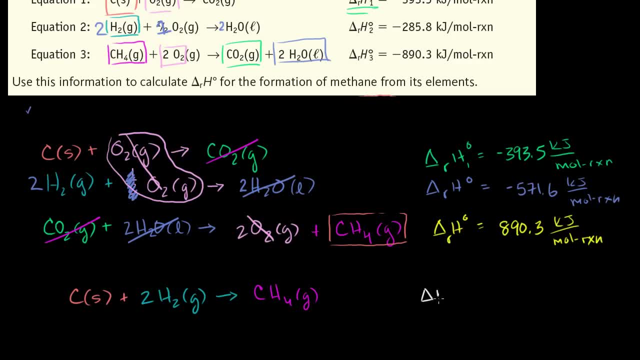 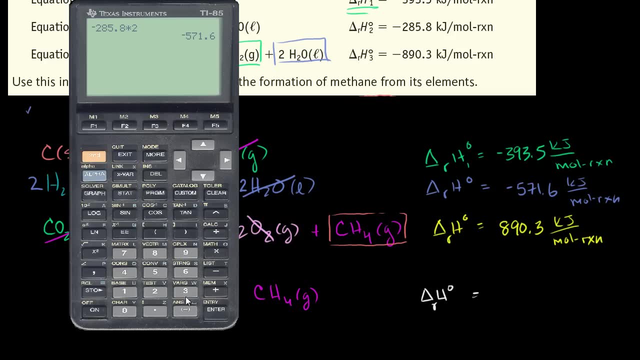 its change in enthalpy of this reaction is going to be the same. It's going to be the sum of these right here. That is Hess's law. So this is the fun part. So we just add up these values right here.